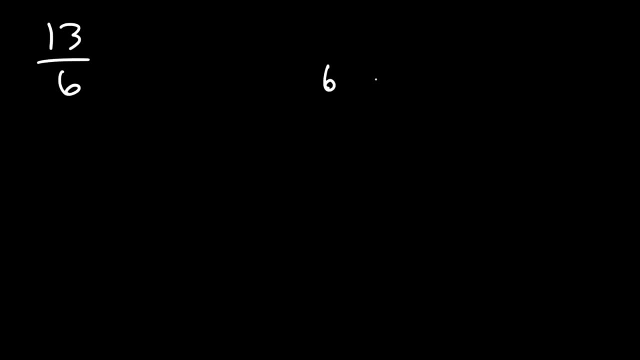 13 over 6.. You can try this if you want to. So how many times does 6 go into 13?? 6 goes into 13 two times. 6 times 2 is 12.. 6 times 2 is 18, which exceeds 13.. 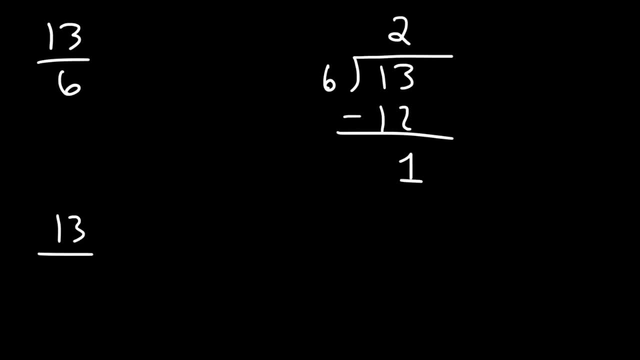 13 minus 12.. 12 is 1., And so we can write our answer as 2 and 1 over 6.. So this is the whole number, And the remainder is the numerator of the mixed number. Now here are two examples that you can try: 21 over 2 and 35 over 12.. Feel free to pause. 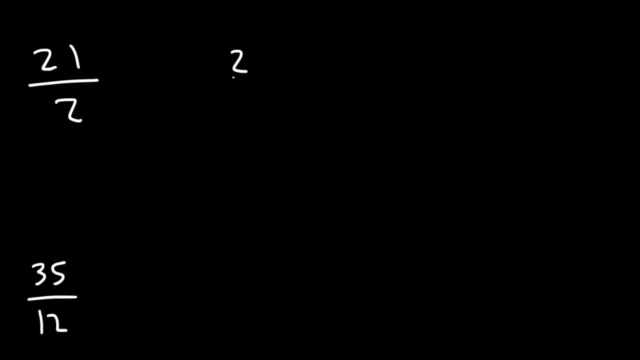 the video and work on those example problems. So let's start with the first one, which I'm going to do. on the right side: How many times does 2 go into 21?? 2 goes into 21. 10 times 2 times 10 is 20 and 21 minus. 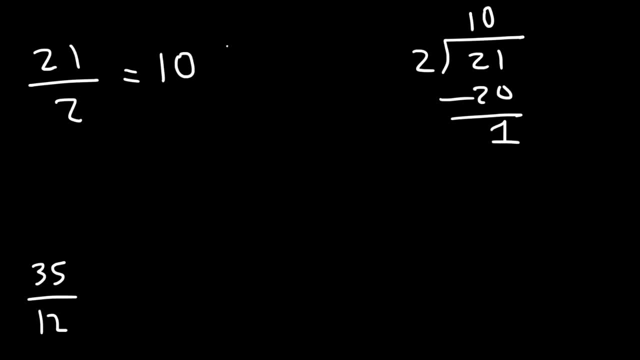 20 is 1.. So the answer is going to be 10 and 1 over 2.. Now, what about the last one? How many times does 12 go into 35?? 12 times 3 is 36.. So that's too much. 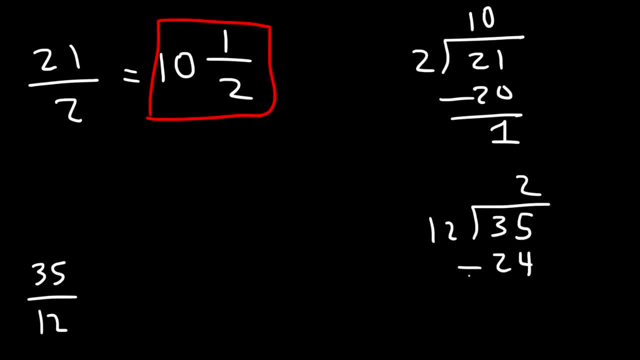 So it's 2.. 12 times 2 is 24, and 35 minus 24 is 11.. So the answer is going to be 2 11 over 12.. So now let's get these same answers using another technique. 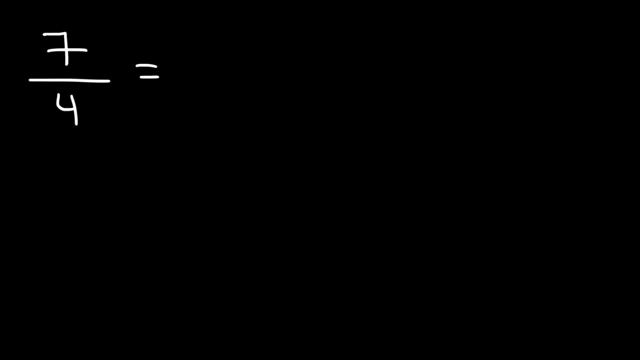 So let's start with 7 over 4.. So what I like to do is break down 7 into two numbers, one of which is divisible by 4.. So 7 is 4 plus 3.. Now the denominator has to be the same when doing this. 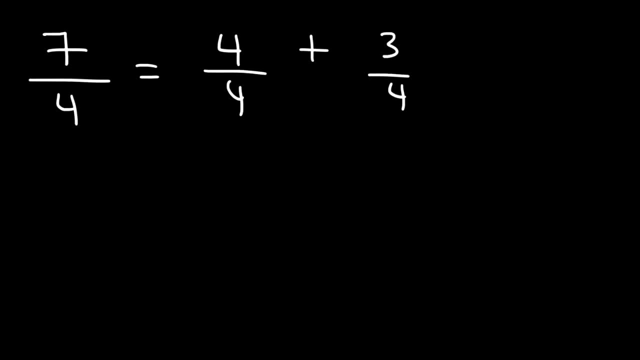 So we can say that 7 over 4 is basically 4 over 4 plus 3 over 4, because 4 plus 3 is 7.. Next, divide: 4 over 4 is 1.. So we have 1 plus 3 fourths, which is the same as 1 and 3 fourths.